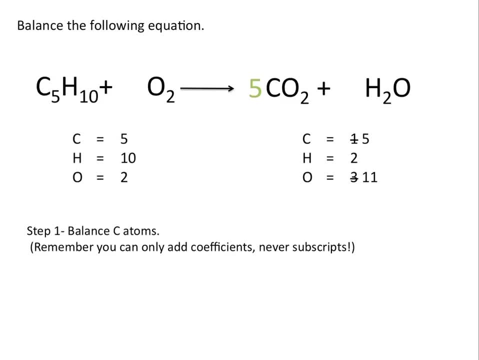 product side, But by putting a five in front of CO2, we've not only changed the number of carbon atoms on the product side to five, but we've also changed the number of oxygen atoms on the product side. So we have five carbon atoms from CO2 and one oxygen atom from H2O, giving us a total of 11 oxygen atoms. 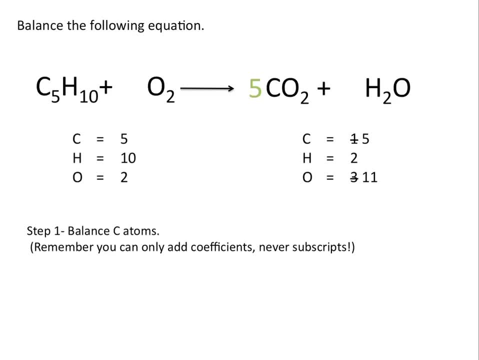 Now let's balance the number of hydrogen atoms, And the reason I'm choosing to balance hydrogen first, before oxygen, is because hydrogen occurs in only one compound on the reactant side and one compound on the product side. So because we have 10 hydrogen atoms on the reactant side and two on the product side, we'll need to put a five. 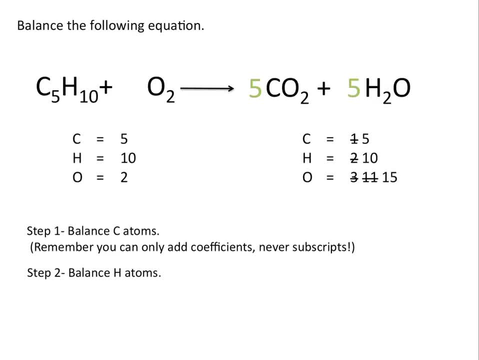 coefficient in front of H2O to give us 10 hydrogen atoms on the product side. But in putting a five in front of H2O, we've not only changed the number of hydrogen atoms on the product side, but we've changed the number of oxygen atoms as well. 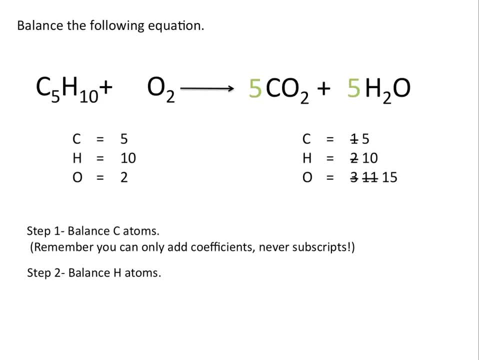 So we now have 10 oxygen atoms from CO2, which we found by taking five times the subscript on oxygen- two to give us 10, but we have an additional five oxygen atoms from H2O, giving us a total number of oxygen atoms of. 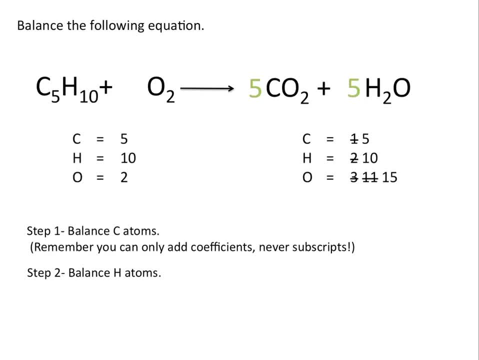 15.. Now we need to balance the number of oxygen atoms. Now you'll see that we have O2 on the reactant side and we have 15 oxygen atoms on the product side that we need to balance. Now putting any coefficient in front of O2 is going to give us an even number of oxygen. 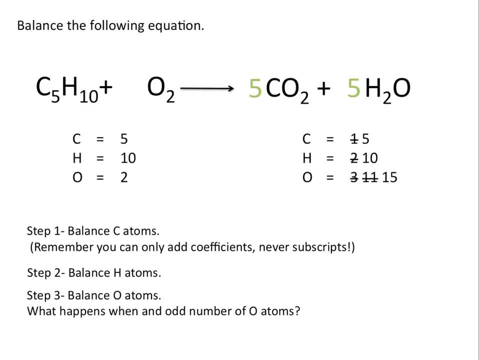 atoms, And so the trick to balancing these combustion reactions is to start by putting a fractional coefficient in front of O2. case we'll choose 15 halves, because 15 halves times the coefficient on O2, which is 2, gives us 15 oxygen atoms on the reactant side, which now balances with the 15 oxygen atoms on the. 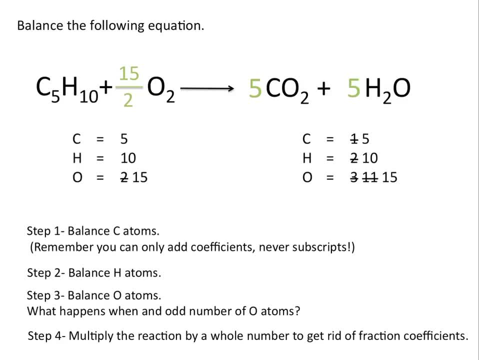 product side. But we can't have a balanced equation with fractions as coefficients. so we need to multiply all of the coefficients in our entire reaction by 2 so that we have all whole number coefficients, And when we do that we'll see that we have 2C5H10 plus. 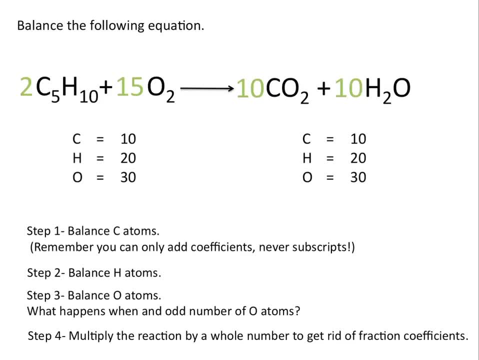 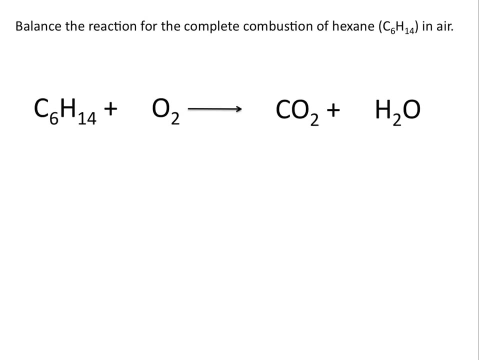 15O2 gives us 10CO2 plus 10H2O, And if you count up the number of carbon hydrogen and oxygen atoms on your reactant side, they will equal the number of carbon hydrogen and oxygen atoms on your product side. Let's try another problem In this reaction. 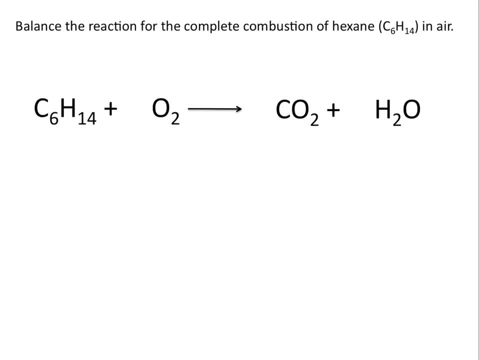 we're combusting hexane, which has the formula C6H14, in air, And the molecule in air that's going to react in this combustion reaction is just O2.. Now hexane and O2 will combust to give us CO2 and H2O. So first let's take inventory of how many of each different type. 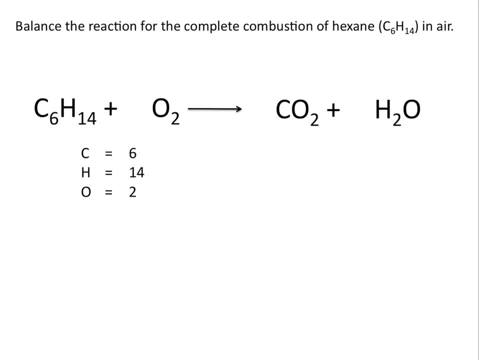 of atom we have on our reactant side and our product side. And then let's start by balancing the components. Let's start with the carbon atoms first. So to balance out the 6 carbon atoms on our reactant side, we need to put the coefficient 6 in front of CO2.. That now gives us 6 carbon. 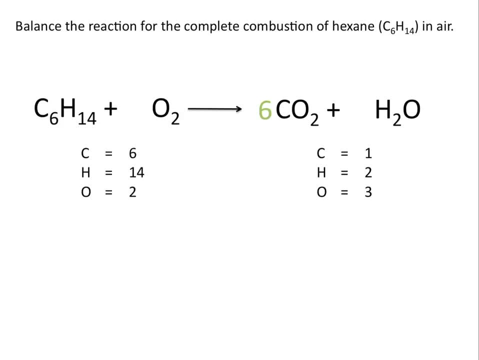 atoms on our product side, But it also increases the number of oxygen atoms on our product side. So we have 12 oxygen atoms from the 6 CO2 molecules, plus 1 oxygen atom from H2O. Let's balance the number of hydrogen atoms next. So we have 14 hydrogen atoms on our 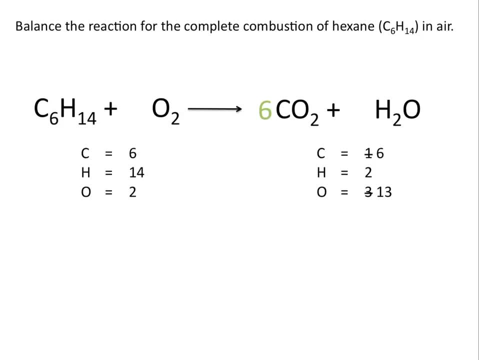 reactant side, And so, in order to have 14 hydrogen atoms on our product side, we need to put the coefficient 7 in front of H2O. That gives us 7 times 2, 14 hydrogen atoms, But it also increases the number of oxygen atoms we have on our product side. So now, 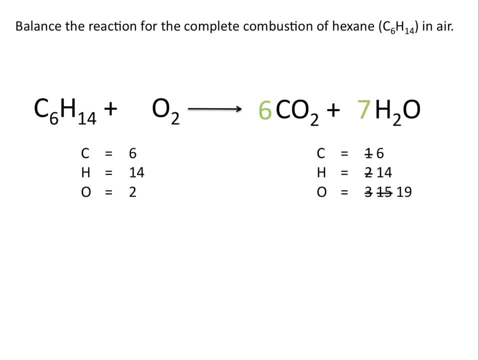 we have 12 oxygen atoms from our product side, So we have 7 times 2, 14 hydrogen atoms. So we have 6 CO2 atoms from our 6 CO2 molecules, plus an additional 7 oxygen atoms from our 7 molecules of H2O, for a total of 19 oxygen atoms. Now, just like in our last example,